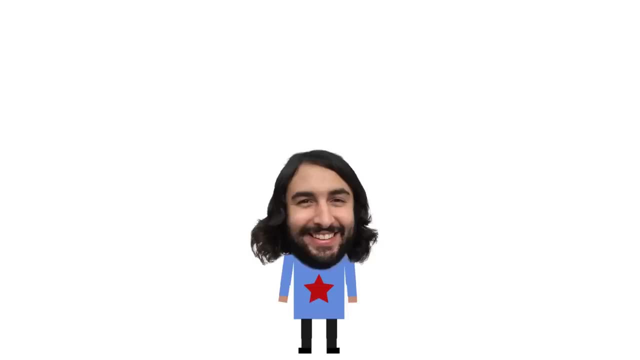 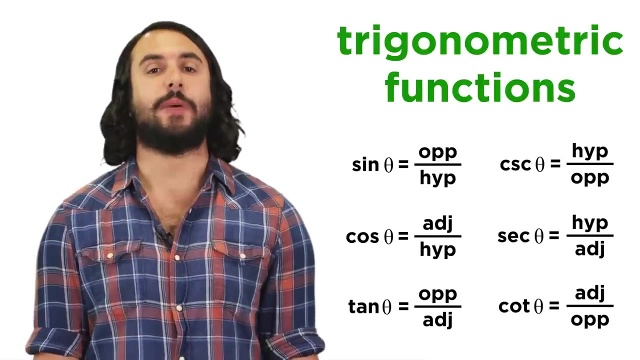 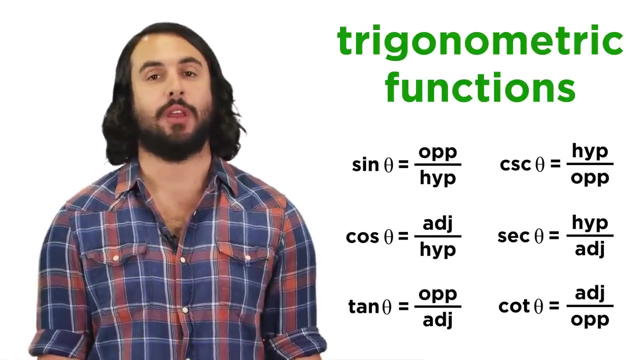 Professor Dave, here let's graph some trig functions. We've just spent some time learning about the six trigonometric functions, as well as how they relate to one another and the unit circle. Just like any other function. we will want to be able to graph them, but there are some. 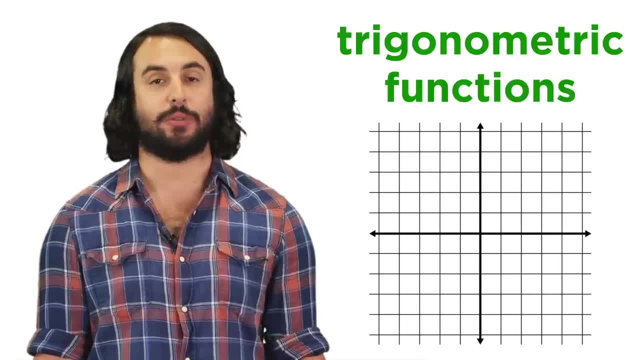 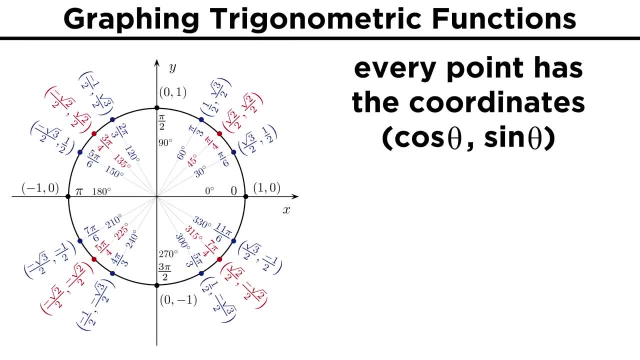 interesting things that we can point out about these functions first. First, let's talk about the domain and range of the functions. Looking back at the unit circle, we know that each point has the coordinates cosine, theta, sine theta. So looking first at sine theta, the domain of this function is the set of all the angles. 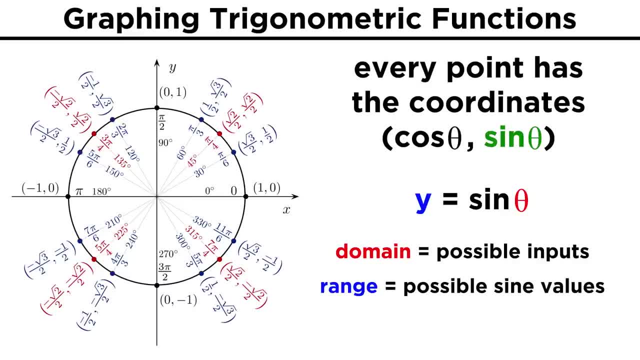 we could plug into this function and the range of the function is all the possible values for sine theta. This means that the domain of sine theta is all real numbers. Since we could plug in any angle, It could be greater than two pi radians. we just end up going around and around indefinitely. 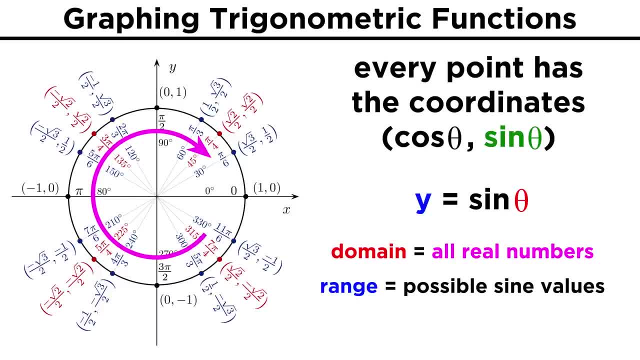 as we approach infinity, And we could also have negative angles. we just go the other way. But the range of the function is negative, one to one inclusive. Sine theta can only have values within this interval, as we can clearly see from the unit. 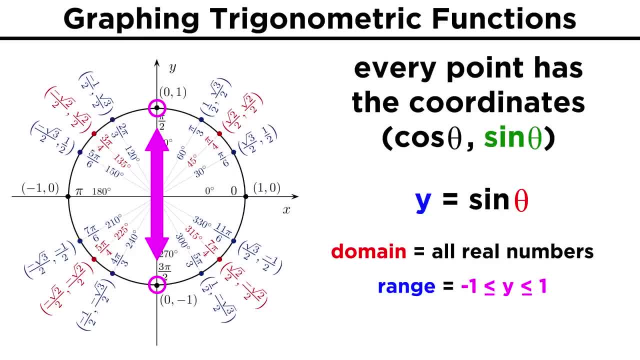 circle, as the Y values of all of these points are equal. So we can only have values within this interval, as we can clearly see from the unit circle, as the Y values of all of these points are equal. The same goes for cosine theta. we could plug in any angle, but if we look at the X, 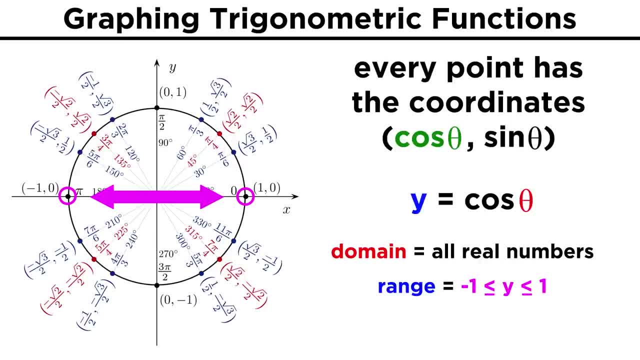 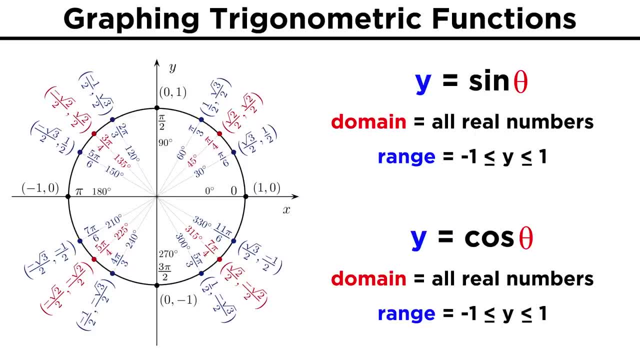 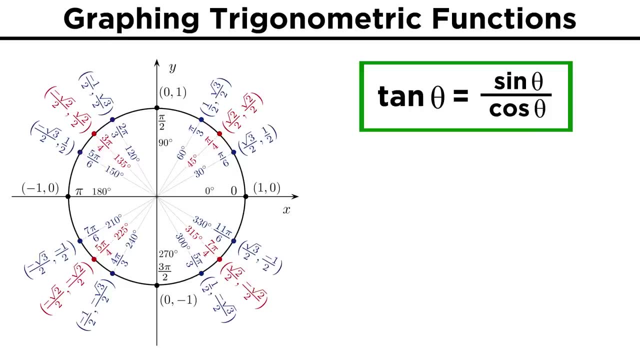 values of these points. they always fall between negative one and one. So both sine and cosine will have a domain of all real numbers and a range of negative one to one Tangent is different because that's sine over cosine And as cosine gets very close to zero in either direction, the function gets very big, approaching 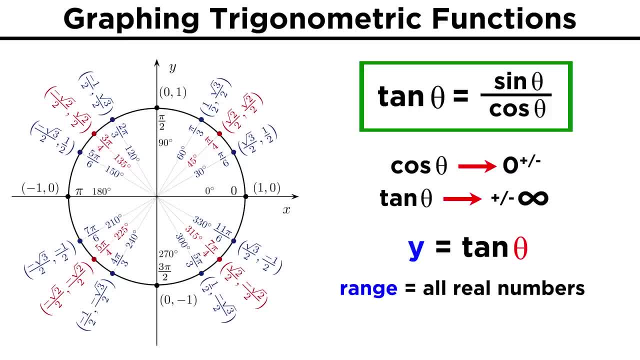 infinity. So the range of tangent theta will be all real numbers. The domain is almost all real numbers. but we can't evaluate tangent when cosine is zero, because anything over zero is undefined. Cosine is zero at half pi and three halves pi. so the domain of tangent theta is all 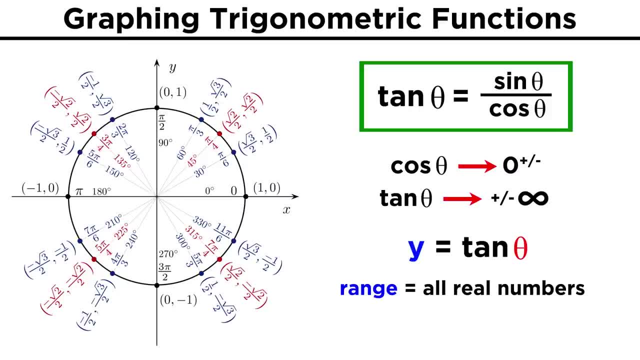 So the range of tangent theta will be all real numbers. The domain is almost all real numbers, but we can't evaluate tangent when cosine is zero, because anything over zero is undefined. Cosine is zero at half pi and three halves pi. So the domain of tangent theta is all real numbers, except half pi, plus or minus multiples. 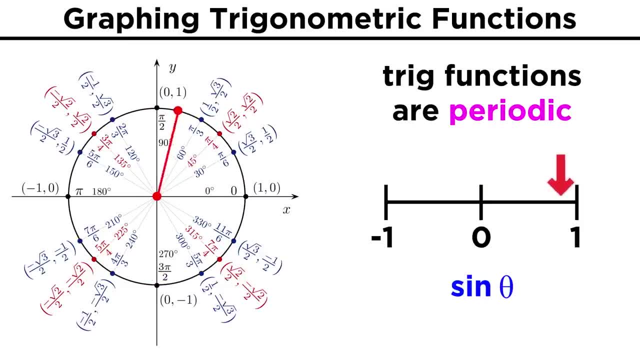 of pi. The other thing we want to understand about these trig functions is that they are periodic. Their values repeat over and over again as we go through each period of the function. The period of these functions is two pi radians, because after two pi radians we are back. 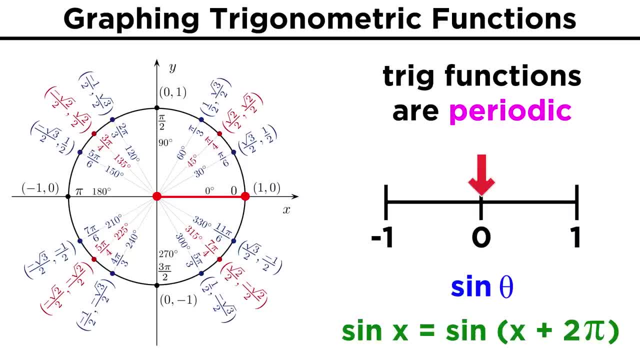 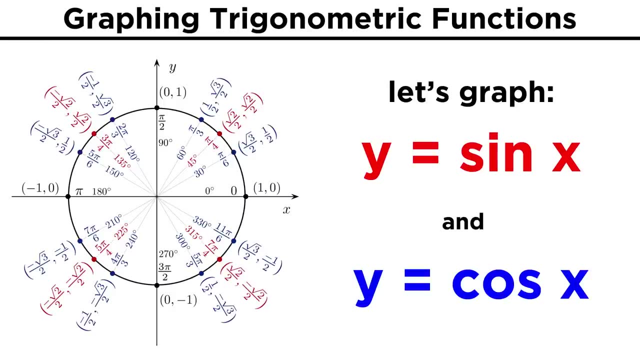 to where we started and all the values repeat. In other words, the sine of X plus two pi is the same as the sine of X. The same goes for cosine. Let's go ahead and graph the sine and cosine functions now, so we can see exactly what. 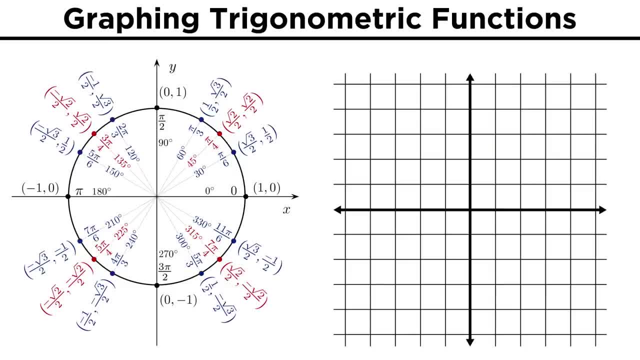 they look like. Let's bring up the coordinate plane and also the unit circle. Looking at the Y coordinates of these points, we can start to plot the graph of Y equals sine X, going in multiples of pi over six. When X is zero, Y is zero. 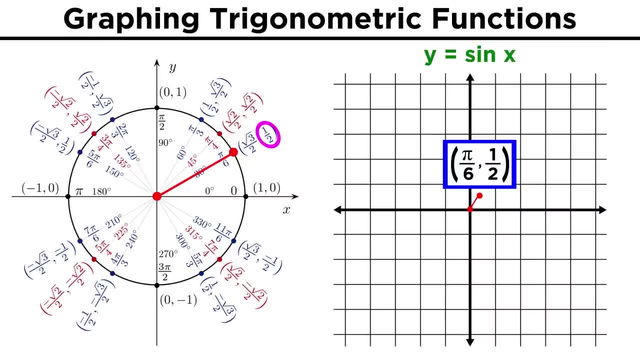 When X is pi over six, Y is one half. When X is pi over three, Y is root three over two. When X is half pi, Y is one. Then, as we move through quadrant two of the unit circle, the sine values start to go back. 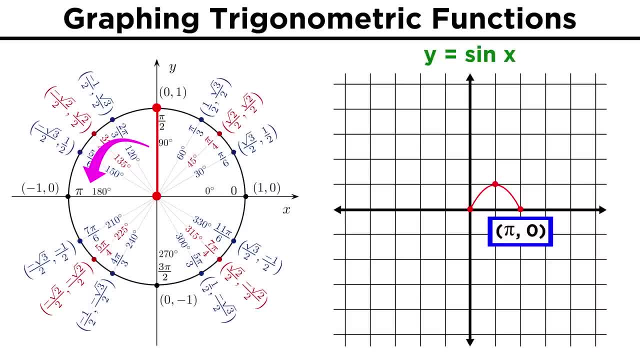 down until we get to X equals pi. Now, as we enter quadrant three, we start to get negative values for the Y coordinate and thus negative values for sine X. These will be the same values as the first two quadrants, just negative until we get. 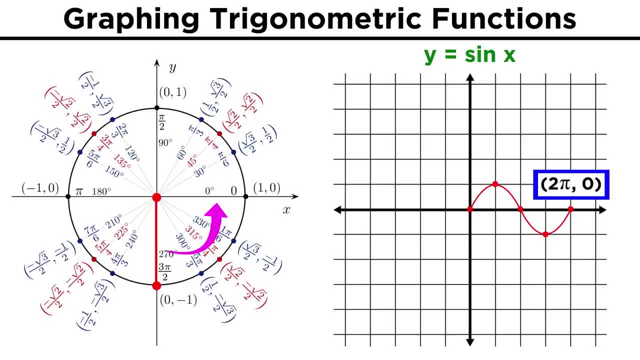 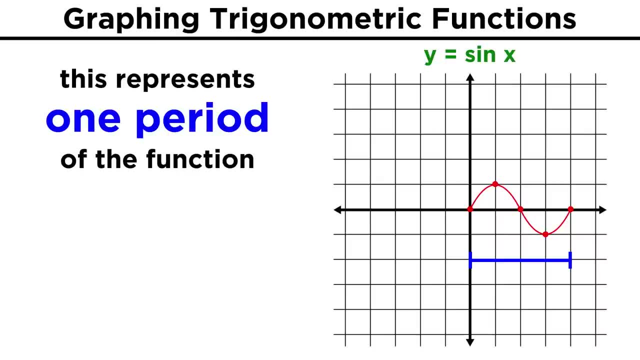 to negative one, And then, moving through the fourth quadrant, we get back to zero. So there is the graph of Y equals sine X, And then we get to two pi radians. it's the same as being at zero, and when we enter, 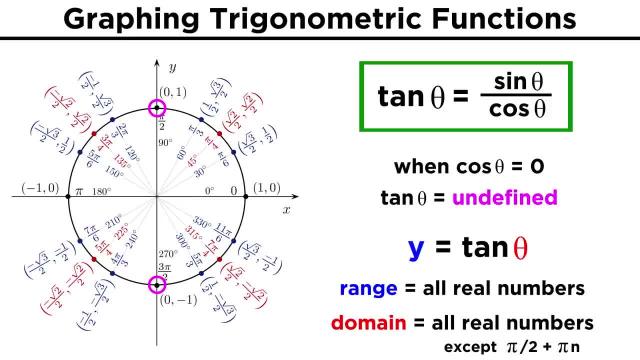 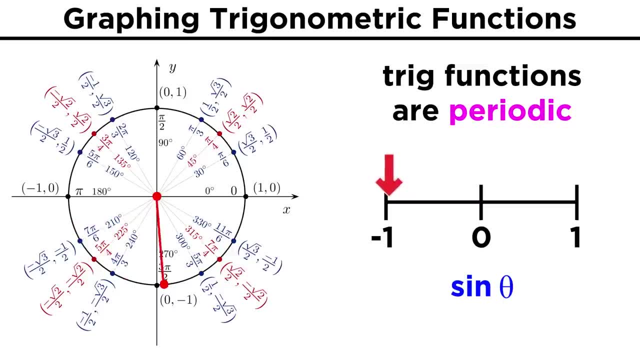 real numbers, except half pi plus or minus multiples of pi. The other thing we want to understand about these trig functions is that they are periodic. Their values repeat over and over again as we go through each period of the function. The period of these functions is two pi radians, because after two pi radians we are back to 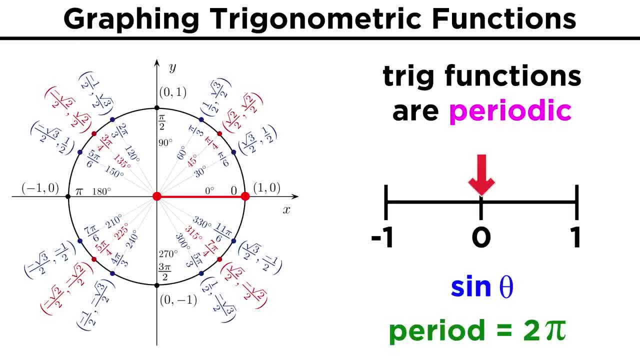 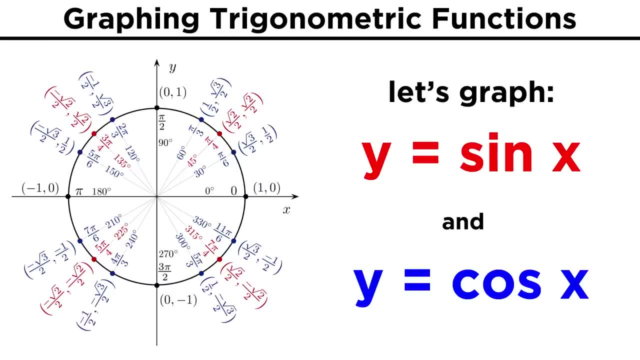 where we started and all the values repeat. In other words, the sine of X plus two pi is the same as the sine of X. The same goes for cosine. Let's go ahead and graph the sine and cosine functions now, so we can see exactly what. 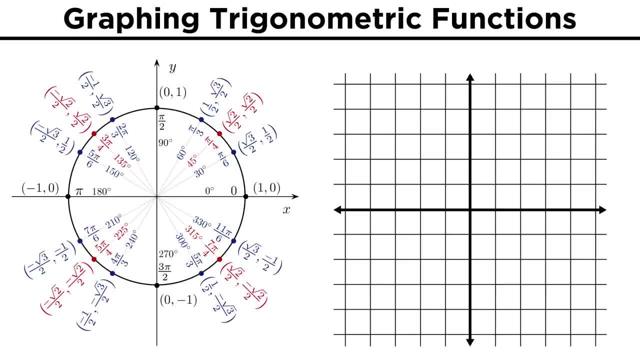 they look like. Let's bring up the coordinate plane and also the unit circle. Looking at the Y coordinates of these points, we can start to plot the graph of Y equals sine X, going in multiples of pi over six. When X is zero, Y is zero. 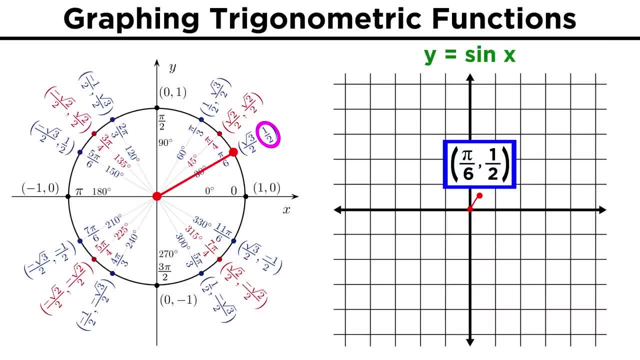 When X is pi over six, Y is one half. When X is pi over three, Y is root three over two. When X is half pi, Y is one. Then, as we move through quadrant two of the unit circle, the sine values start to go back. 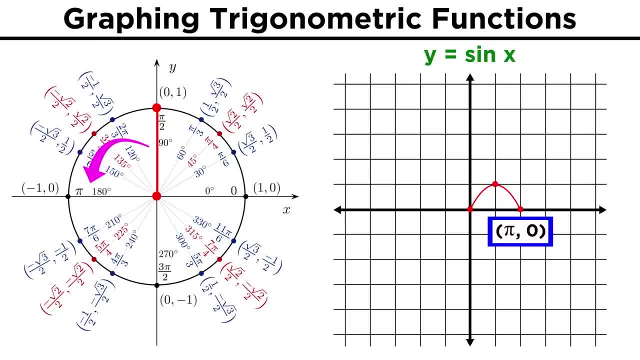 down until we get to X equals pi, where Y is again zero. Now, as we enter quadrant three, we start to get negative values for the Y coordinate and thus negative values for sine X. These will be the same values as the first two quadrants, just negative until we get. 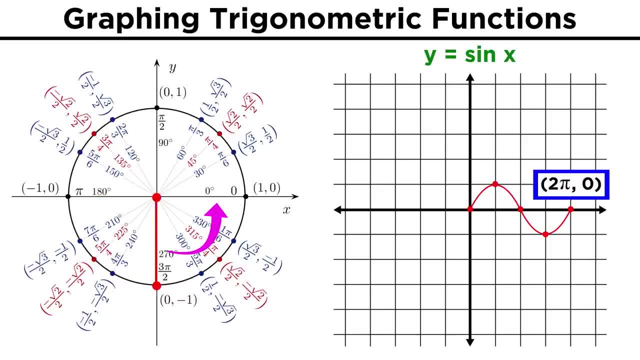 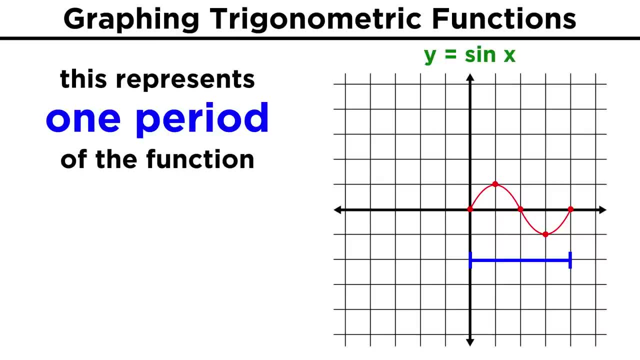 to negative one, And then, moving through the fourth quadrant, we get back to zero. So there is the graph of Y equals sine X for one period of the function. Once we get to two pi radians, it's the same as being at zero, and when we enter another, 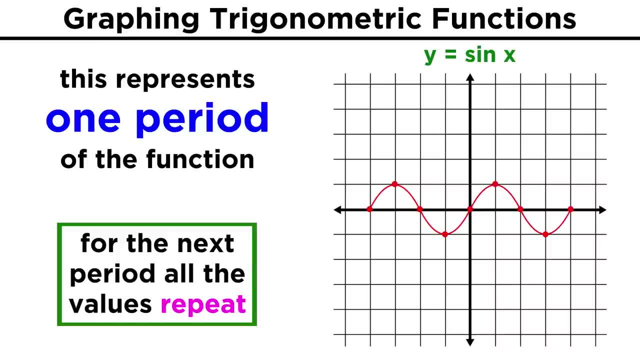 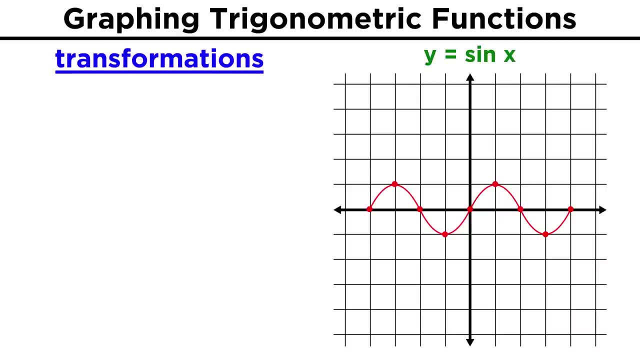 period of the function, all of the values will repeat. That's what makes this a periodic function. If we graph multiple periods of the function, it looks like this and we can clearly see its cyclical nature. How can we manipulate this function? 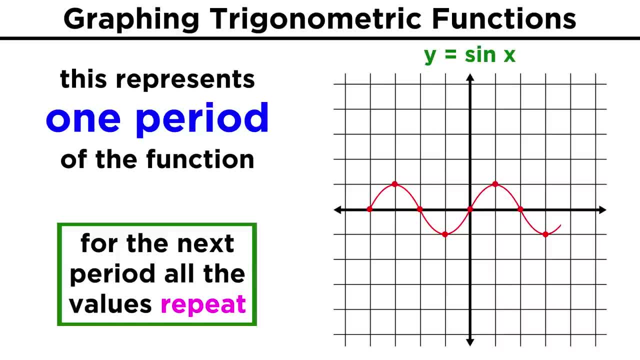 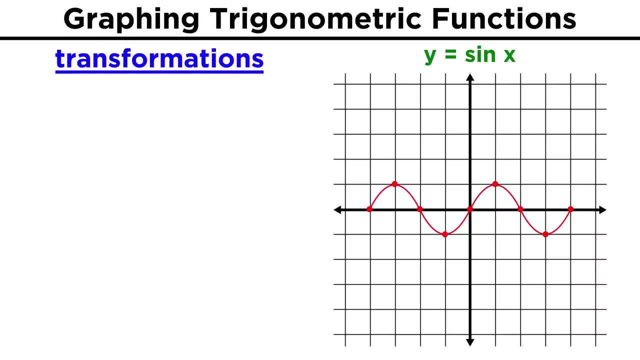 another period of the function, all of the values will repeat. That's what makes this a periodic function. If we graph multiple periods of the function, it looks like this and we can clearly see its cyclical nature. How can we manipulate this function? 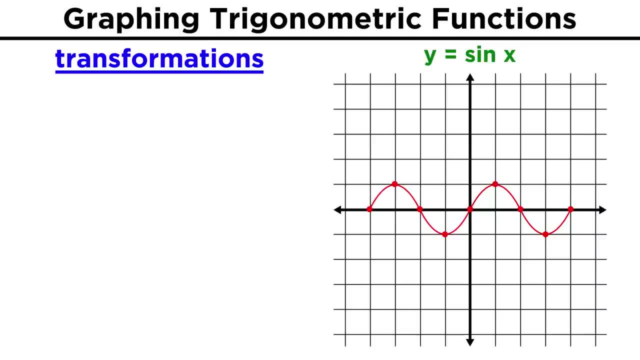 Well, we can apply any of the transformations we learned in our previous class. We can apply any of the transformations we learned in our previous class. We can apply any of the transformations we learned in our previous class. If we put a coefficient here, that will stretch or shrink the function, which will change. 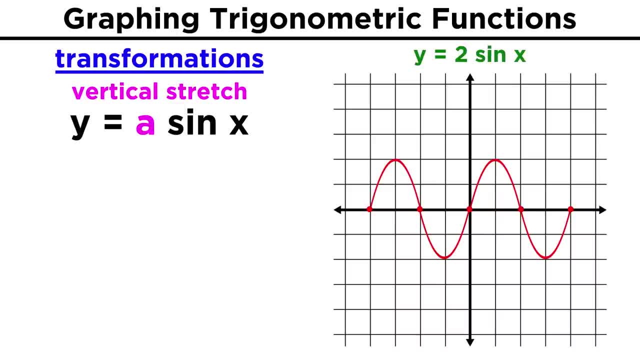 the amplitude of the function. Y equals two sine. X will look the same, except that all the values are doubled. so we are cycling between two and negative two. If the coefficient is negative, it reflects everything across the X axis, which looks like this: 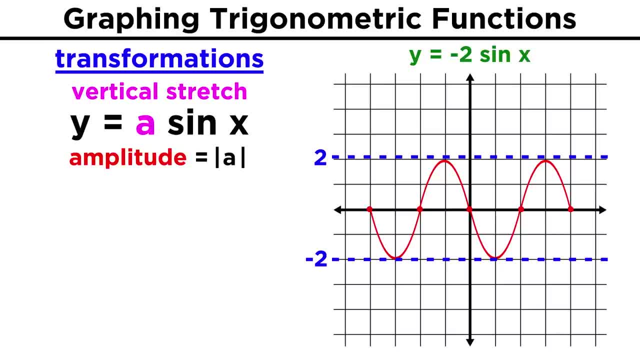 In this way, for any function in the form Y equals two, it will look like this: If the coefficient is negative, it reflects everything across the X axis, which looks like this: In this way, for any function in the form Y equals A sine X, the amplitude will be equal. 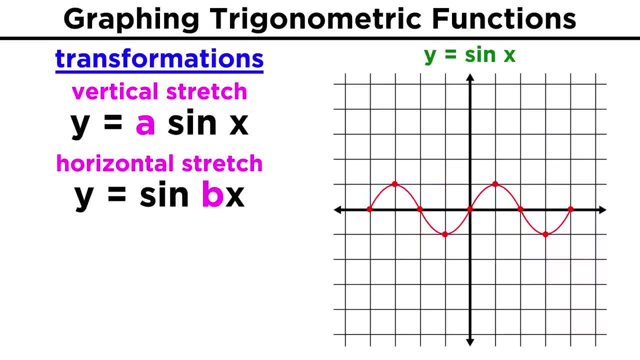 to the absolute value of A. If instead there is a coefficient operating on X, that would be a horizontal stretch. as Y equals sine of two. X would mean that the function will rise and fall at twice the normal rate. This would mean that the period of this function is pi instead of two pi and in fact, for 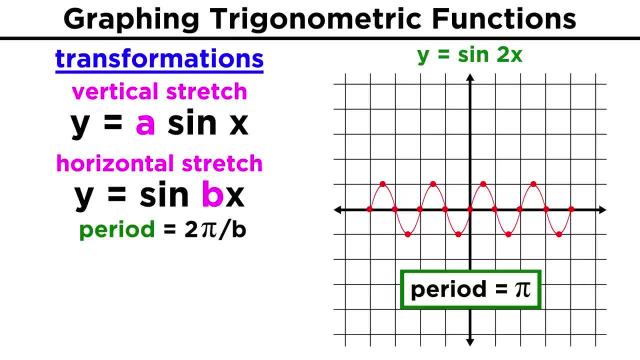 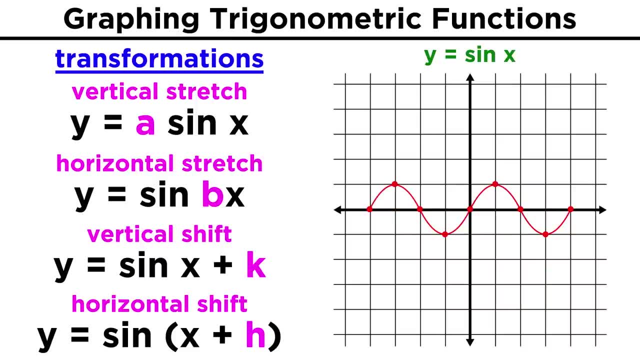 any function in the form of Y equals A sine BX. the period is two pi over B. Lastly, we can have vertical or horizontal shifts. If we have a term that is being added to the function, that's a vertical shift, just like we saw with parabolas. 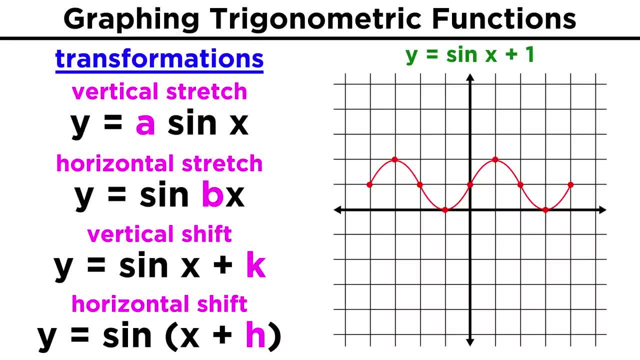 Y equals sine X plus one will just shift everything up one. If instead we have some number inside the function, it will look like this: Y equals sine X plus one will just shift everything up one If instead we have some number inside the function. that's a vertical shift, just like we saw with parabolas. 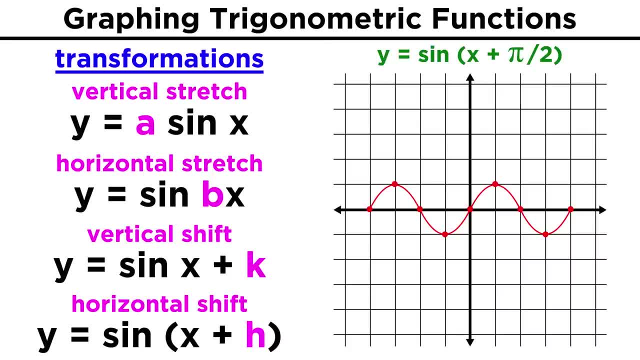 If instead we have some number inside the function like Y equals sine of the quantity X plus half pi, this whole thing will shift half pi to the left. If instead we have some number inside the function, that's a vertical shift, just like. 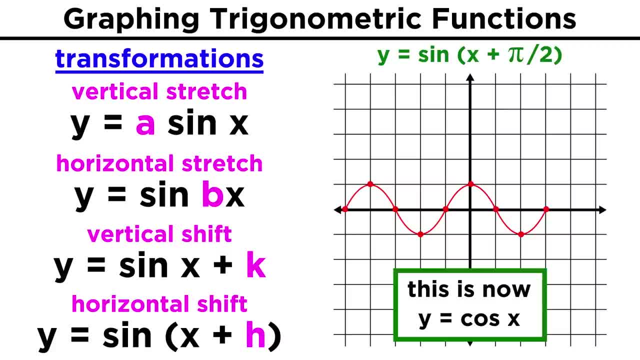 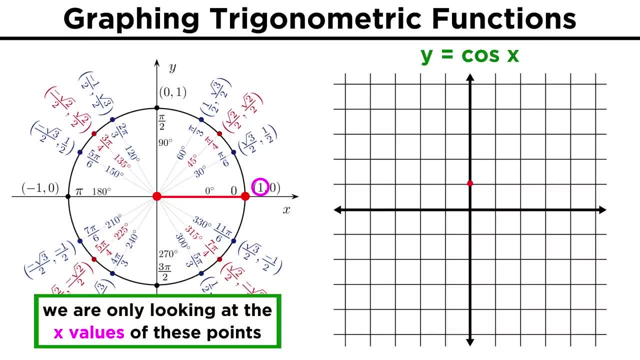 we saw with parabolas. As it happens, we have just generated the graph- for Y equals cosine X. If instead we have some number inside the function, that's a horizontal shift, just like we saw with parabolas. This will make sense if we refer to the unit circle again and see that the cosine of zero. 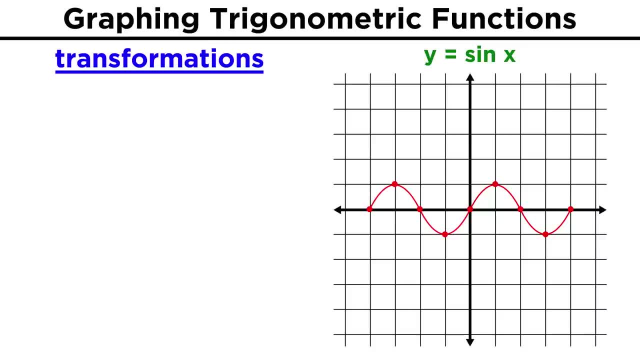 Well, we can apply any of the transformations we learned in algebra. If we put a coefficient here that will stretch or shrink the function, which will change the amplitude of the function. Y equals two sine. X will look the same, except that all the values are doubled. so we are. 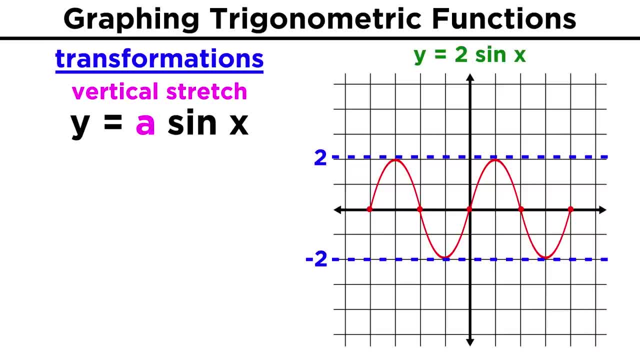 cycling between two and negative two. If the coefficient is negative, it reflects everything across the X axis, which looks like this: In this way, for any function in the form Y equals sine X, it will look like this: For any function in the form Y equals A sine X, the amplitude will be equal to the absolute. 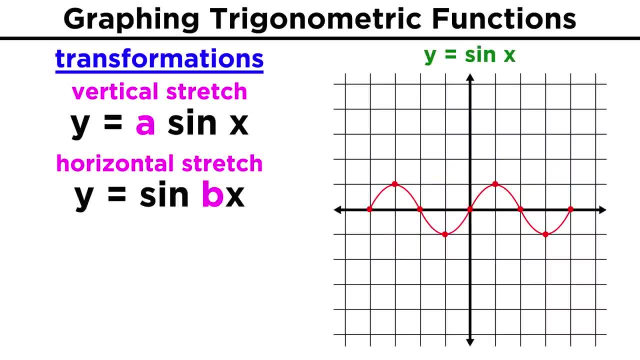 value of A. If instead there is a coefficient operating on X, that would be a horizontal stretch. as Y equals sine of two X would mean that the function will rise and fall at twice the normal rate. This would mean that the period of this function is pi instead of two pi and in fact, for 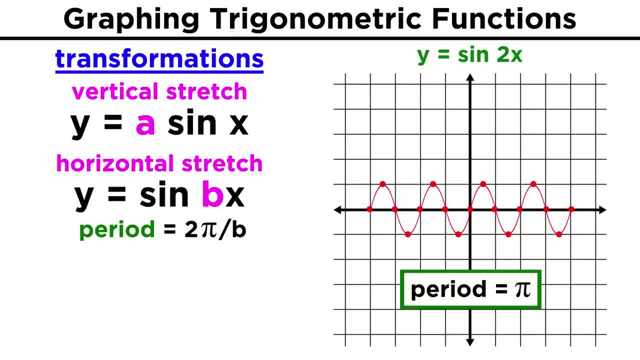 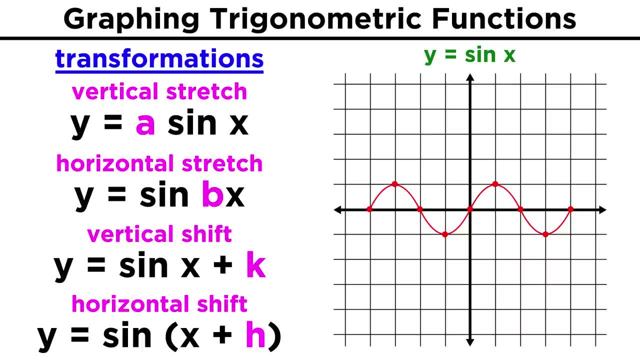 any function in the form of Y equals A sine X, the amplitude will be equal to the absolute value of A. For any function in the form Y equals A sine BX, the period is two pi over B. Lastly, we can have vertical or horizontal shifts. 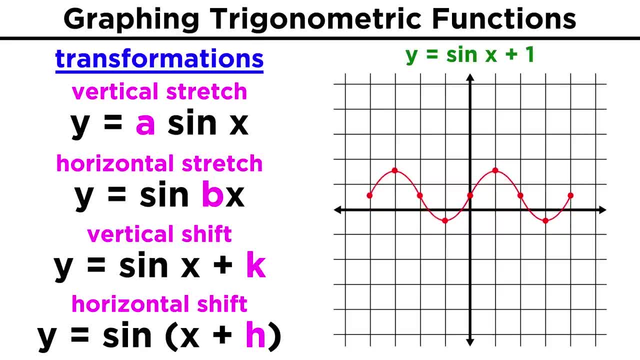 If we have a term that is being added to the function, that's a vertical shift, just like we saw with parabolas. Y equals sine X plus one will just shift everything up one. If instead we have some number inside the function like Y equals sine of the quantity. 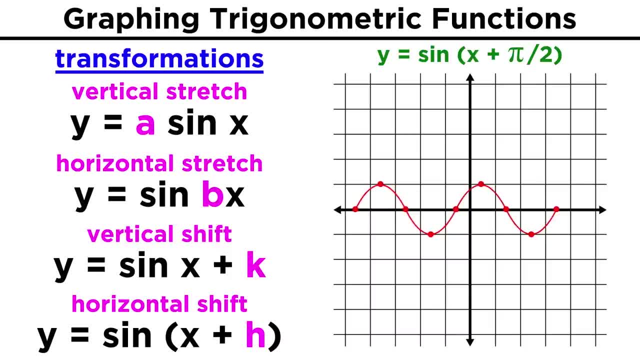 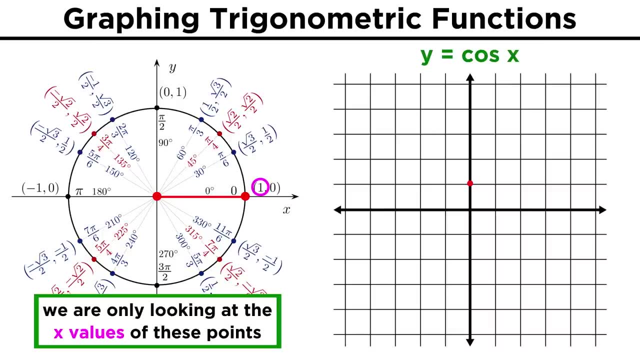 X plus half pi, this whole thing will shift half pi to the left. As it happens, we have just generated the graph, for Y equals cosine X. This will make sense if we refer to the unit circle again and see that the cosine of zero. 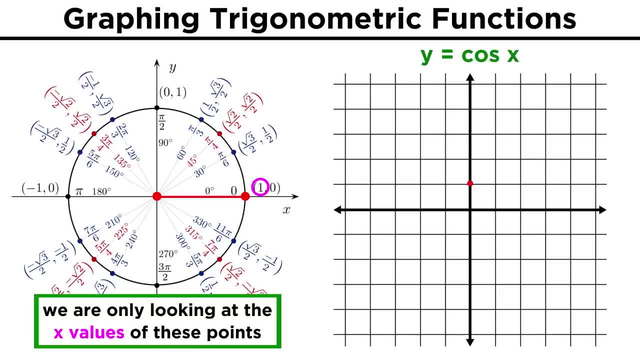 is one. That means the function must start up here. Then the cosine decreases until we get to zero at half pi, then goes towards negative one at pi, then it's back to zero at three halves pi and then up to one at two pi. 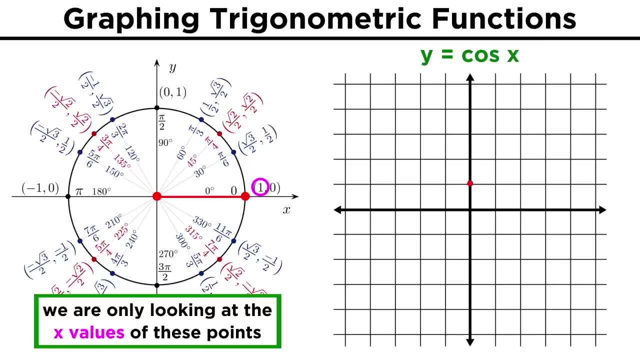 is one. That means the function must start up here. then the cosine decreases until we get to zero at half pi. at half pi then goes towards negative one at pi. then it's back to zero at three halves pi and then up to one at two pi, after which things repeat. 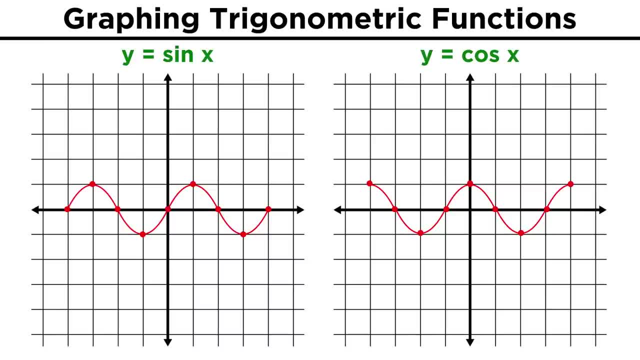 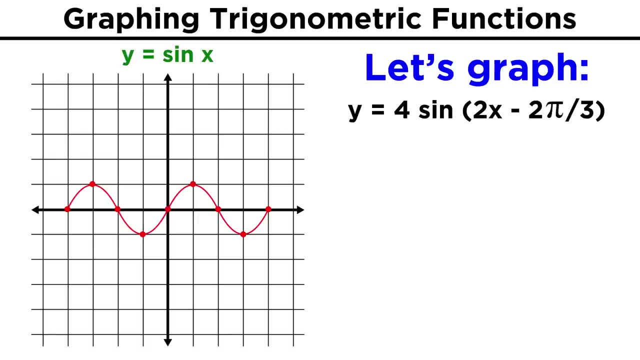 So the graphs for sine and cosine are extremely similar. they are just slightly shifted and all of the transformations we used for sine x will apply to cosine as well. Let's use what we've just learned to graph one period of four sine of the quantity. 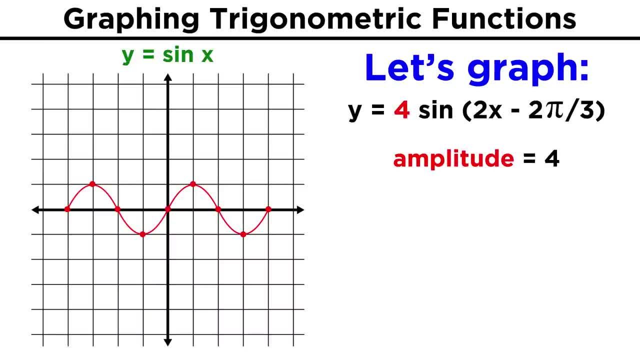 two x minus two thirds pi. First let's find the amplitude. We can get that from this number here, which is four, so the function will move between negative four and four. Then let's find the period. That will be two pi over this term, so the period will be equal to pi. 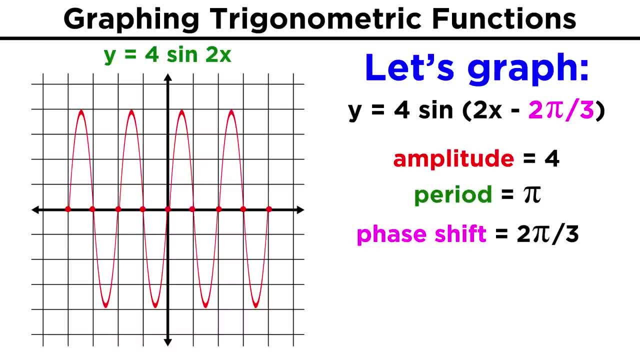 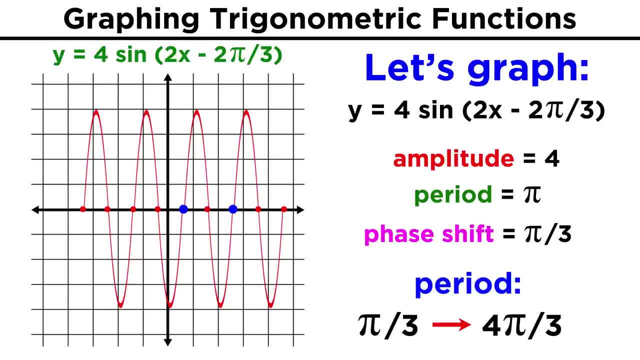 Then we find the function, The phase shift. This term would mean that the whole thing is shifted two thirds pi to the right from the origin. but we have to divide that by this number, since this is causing things to contract. so that leaves us with pi over three. 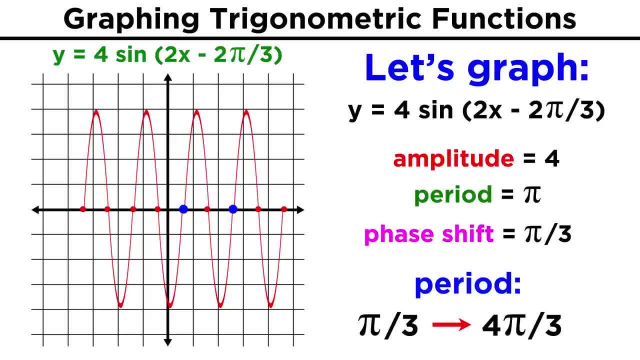 So the period will start at one third pi and end at four thirds pi, going up to four and then down to negative four before coming back to zero. We can find the x-coordinates of the equation. We can find the x-coordinates of these key points as well. we just have to split the. 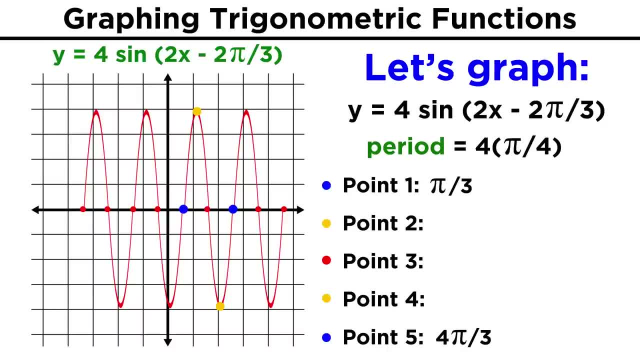 period up into four parts. That gives us a quarter pi, and we just add quarter pi successively, starting with a third pi to get all the x-coordinates. To do that we need a common denominator, which will be twelve, and then we combine and reduce. 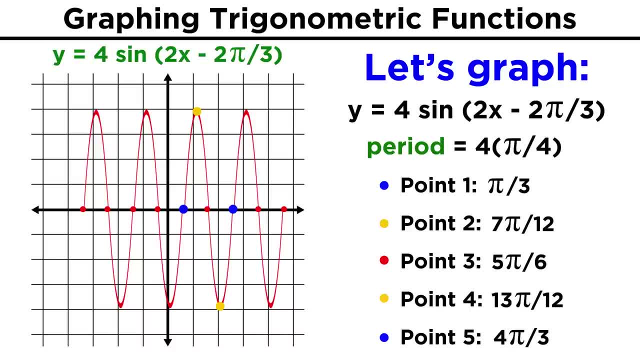 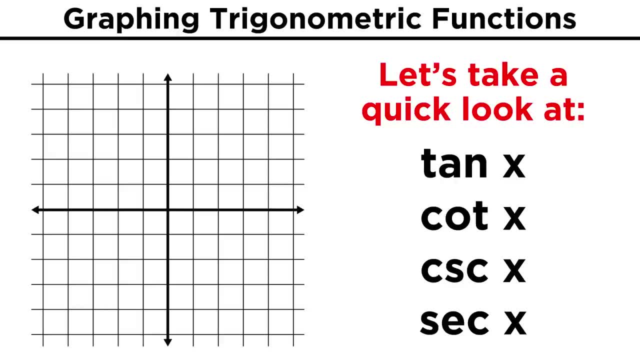 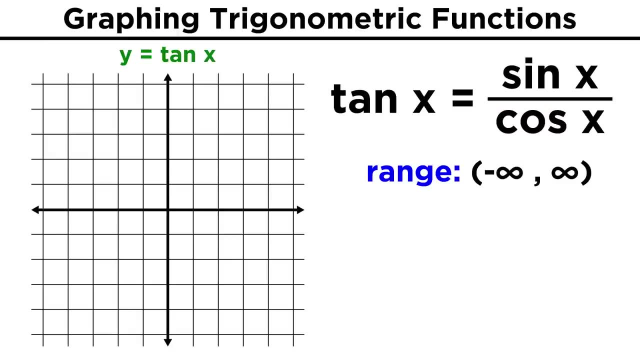 using the rules we already learned for adding fractions. Let's do that Before we move on from this subject. let's just quickly look at the graphs of the other trig functions so that we know what they look like. Tangent looks quite a bit different because the range is no longer negative one to one. 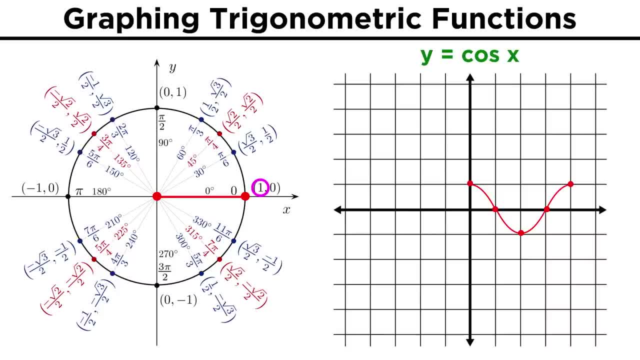 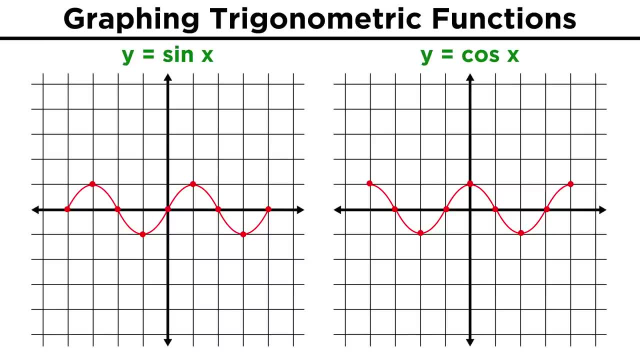 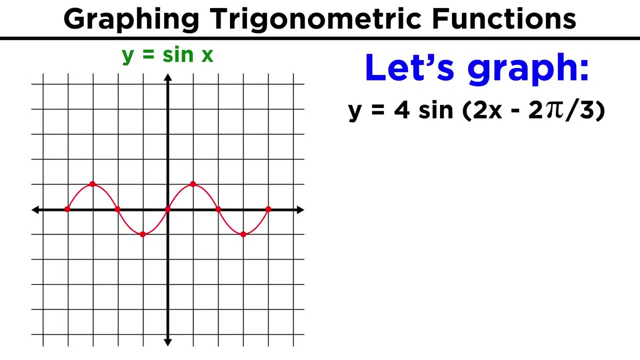 after which things repeat. So the graphs for sine and cosine are extremely similar. they are just slightly shifted, and all of the transformations we used for sine X will apply to cosine as well. Let's use what we've just learned to graph one period of four sine of the quantity X. 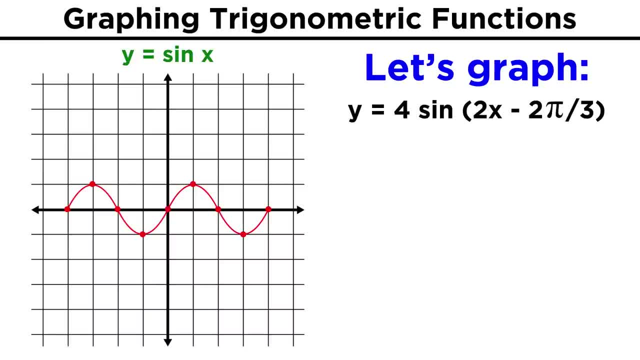 Let's use what we've just learned to graph one period of four sine of the quantity X. Let's use what we've just learned to graph one period of four sine of the quantity X minus two thirds pi. First let's find the amplitude. 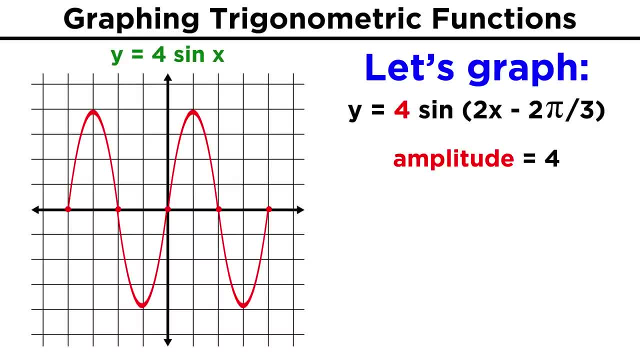 We can get that from this number here, which is four. so the function will move between negative four and four. Then let's find the period. That will be two pi over this term, so the period will be equal to pi. Then we find the phased shift. 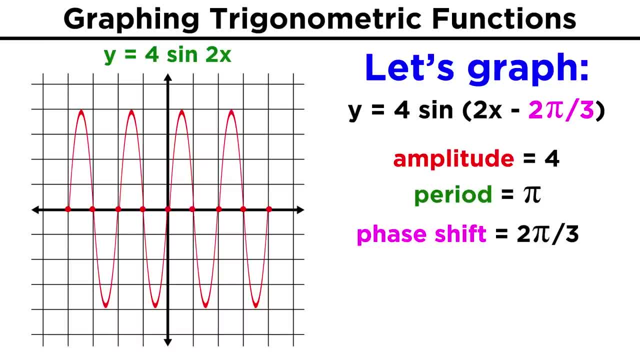 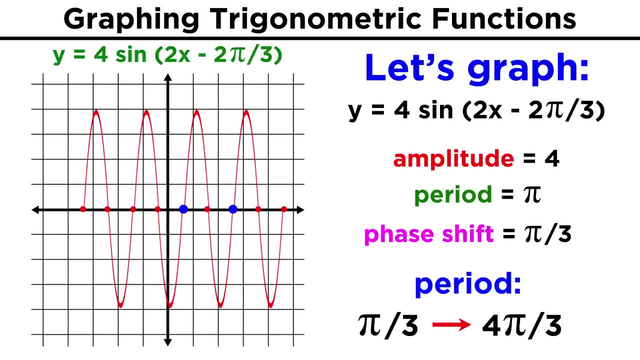 This term would mean that the whole thing is shifted two thirds pi to the right from the origin. but we have to divide that by this number, since this is causing things to contract. so that leaves us with pi over three. So the period will start at one third pi and end at four thirds pi, going up to four. 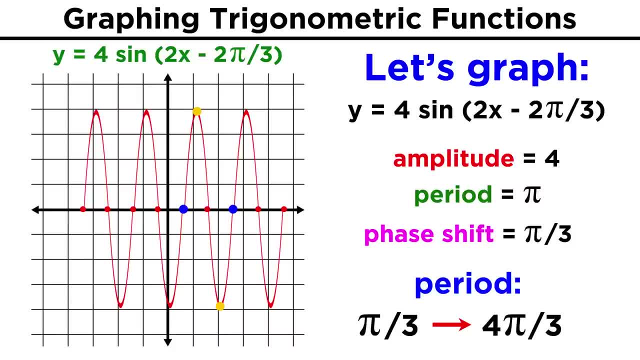 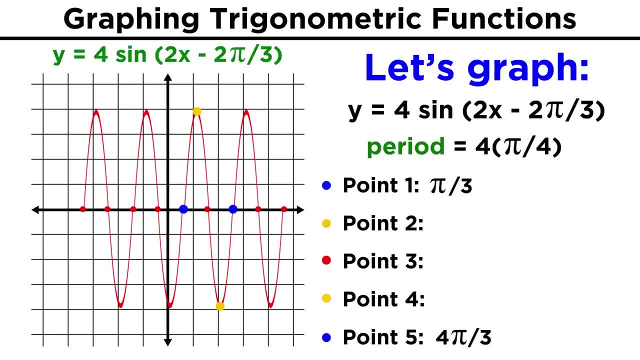 and then down to negative four before coming back to zero. We can find the X coordinates of these key points as well. we just have to split the period up into four parts. That gives us a quarter pi, and we just add quarter pi successively, starting with a third. 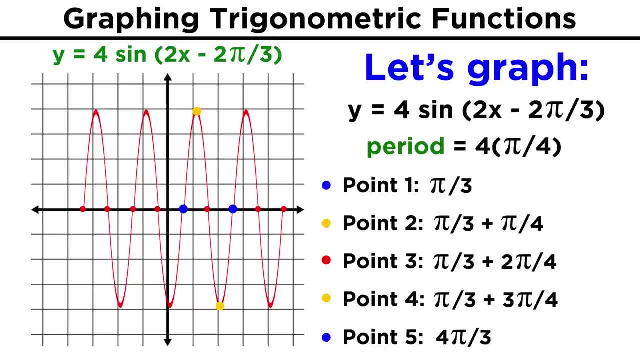 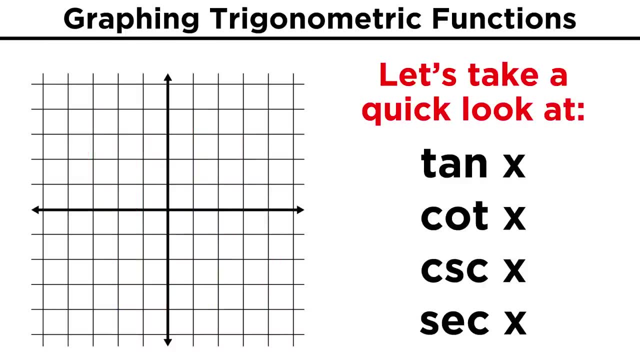 pi to get all the X coordinates. To do that, we need a common denominator, which will be twelve, and then we combine and reduce using the rules we already learned for adding fractions. Before we move on from this subject, let's just quickly look at the graphs of the other 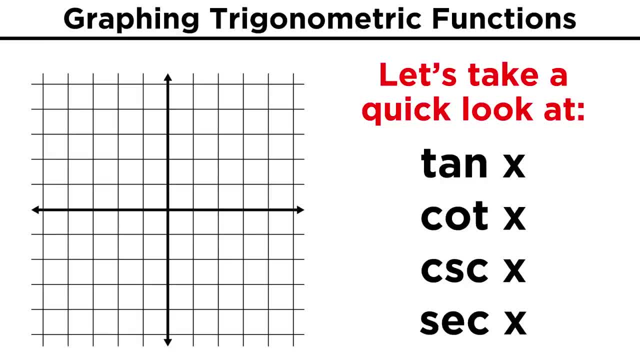 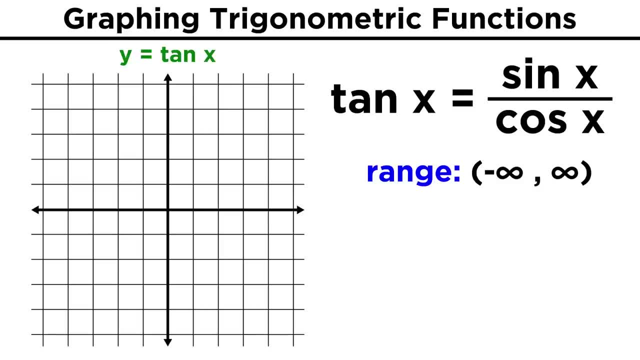 trig functions so that we know what they look like. Tangent looks quite a bit different because the range is no longer negative one to one, like for sine and cosine. Instead, this function approaches positive and negative infinity, as cosine values approach zero. and when cosine is zero, tangent is undefined. so we have a series of vertical. 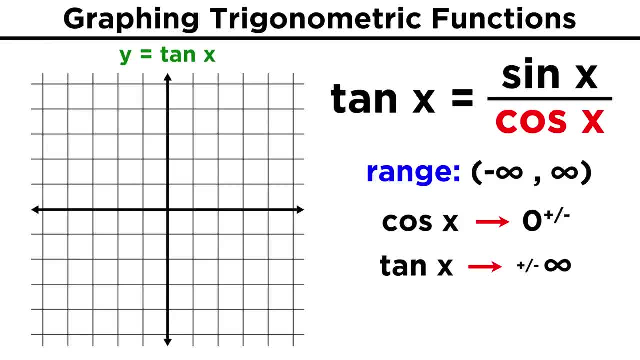 like for sine and cosine. Instead, this function approaches positive and negative infinity, as cosine values approach zero. and when cosine is zero, tangent is undefined. so we have a series of vertical asymptotes. Here is the graph: for y equals tangent x. 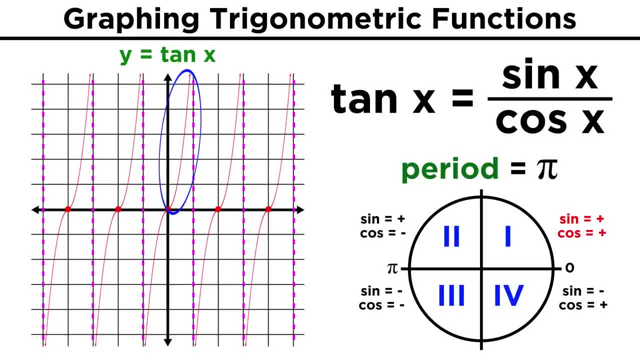 It has a period of pi, because tangent values from quadrant one, where sine and cosine are both positive, come back again in quadrant three, where sine and cosine are both negative. Likewise, tangent values in quadrant two, which are positive over negative, come back. 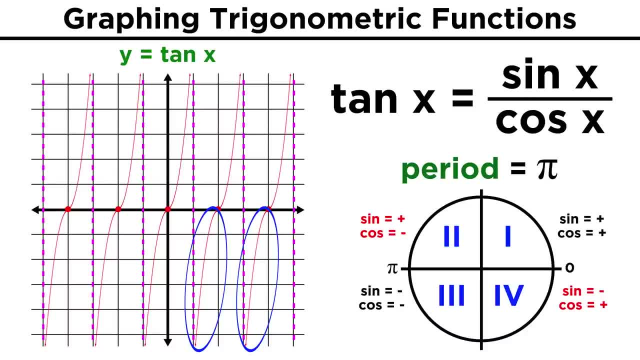 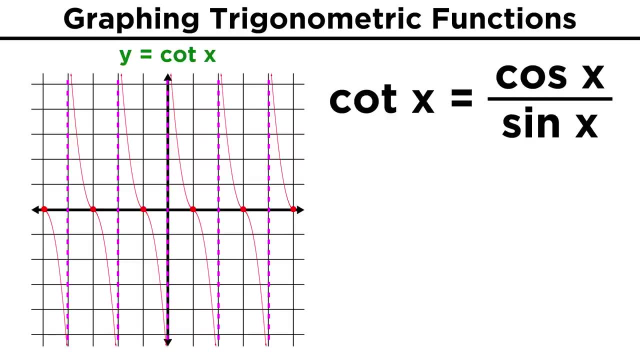 in quadrant four, where it's negative over positive. This function can be transformed in all the same ways that we saw for sine and cosine. Cotangent will be similar but as it is the reciprocal of tangent, it's a little different, falling to the right instead of rising, and shifted slightly since the X values that originally. 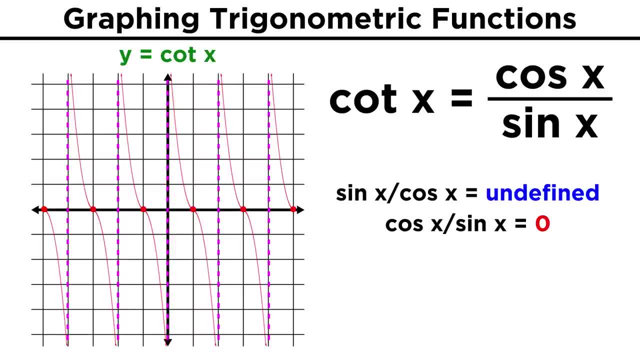 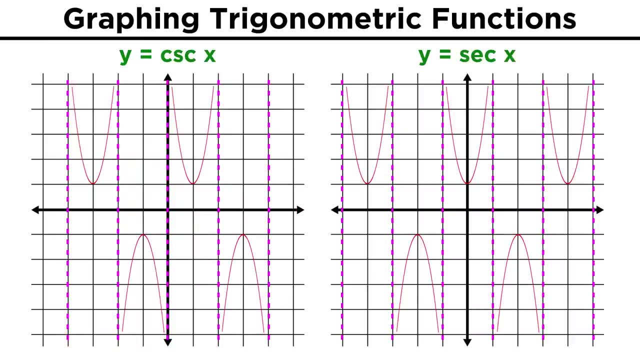 generated asymptotes will now generate Y values of zero, as one over infinity is zero, and the points that originally had Y values of zero will now contain asymptotes, as one over zero is undefined. Cosecant and secant will also look a little funny, as all the points where the sine and 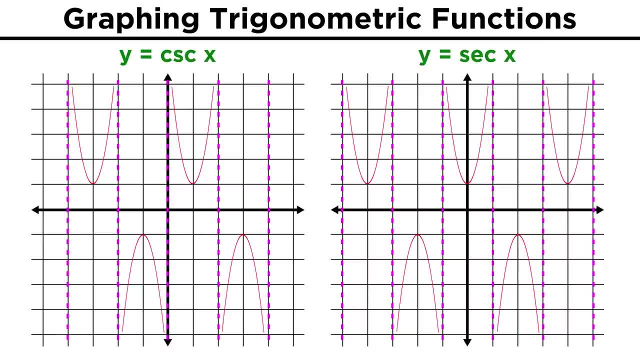 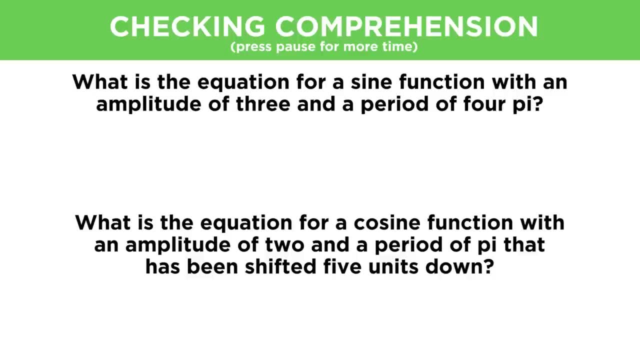 cosine equal zero will now be asymptotes for their reciprocal functions, again, because one over zero is undefined. The transformations for all these graphs are exactly what you would expect, so, having gone over this already, let's check comprehension. Thanks for watching, guys. 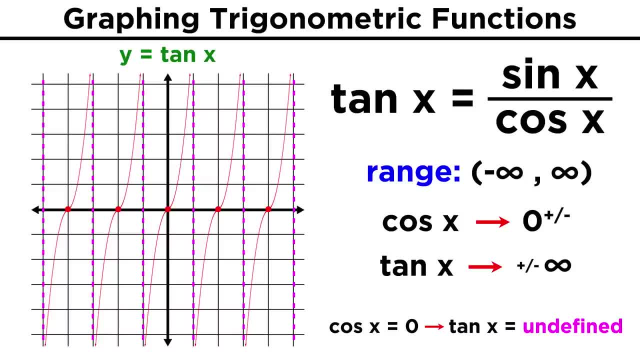 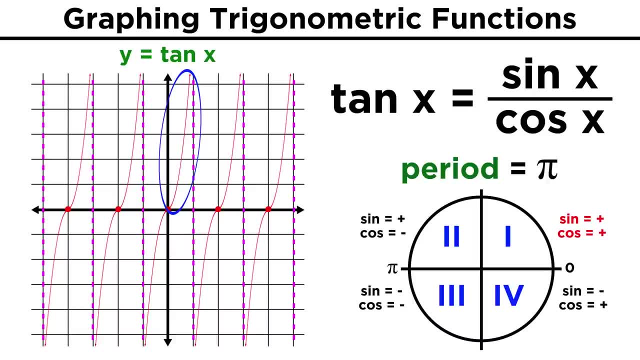 asymptotes. Here is the graph for: Y equals tangent X. It has a period of pi over three. It has a period of pi because tangent values from quadrant one, where sine and cosine are both positive, come back again in quadrant three, where sine and cosine are both negative. 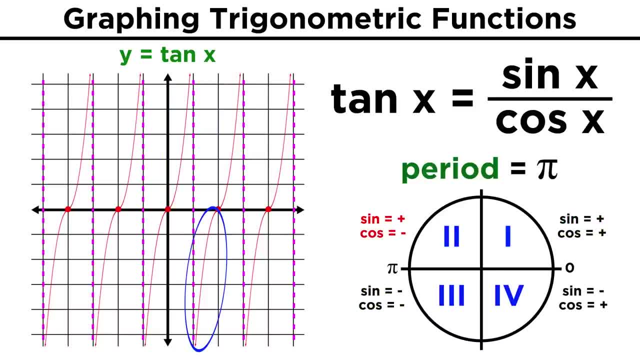 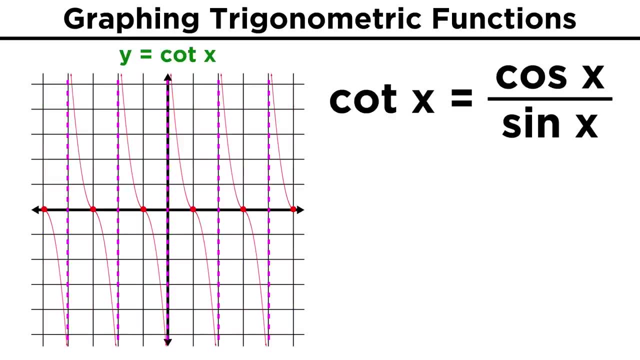 Likewise, tangent values in quadrant two, which are positive over negative, come back in quadrant four, where it's negative over positive. This function can be transformed in all the same ways that we saw for sine and cosine. Cotangent will be similar, but as it is the reciprocal of tangent, it's a little different. 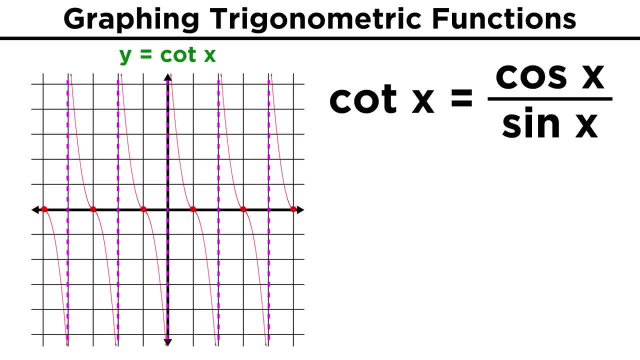 falling to the right instead of rising, and shifted slightly, since the X values that originally generated asymptotes will now generate Y values of zero, as one over infinity is zero and the points that originally had Y values of zero will now contain asymptotes as one over 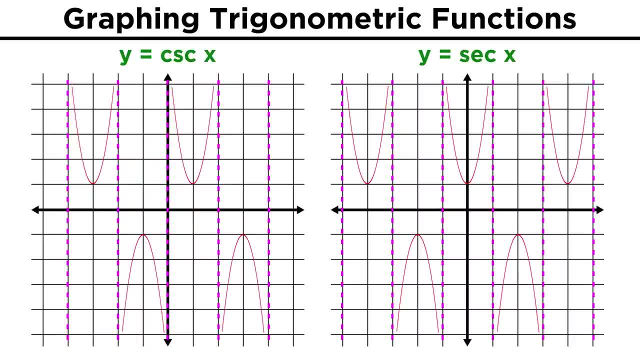 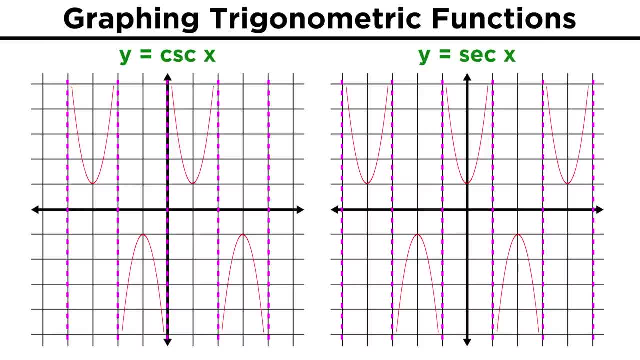 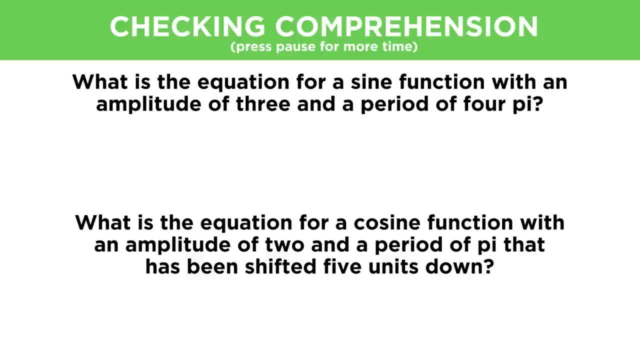 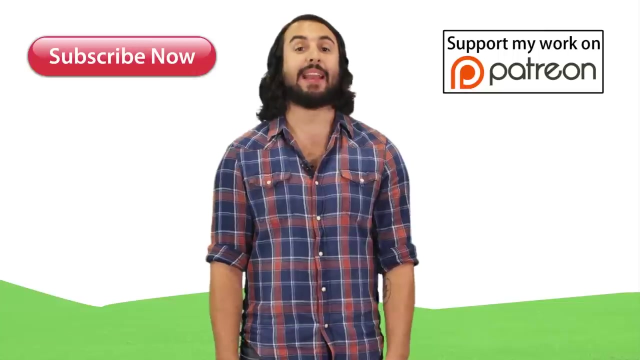 one over zero is undefined. The transformations for all these graphs are exactly what you would expect, so, having gone over this already, let's check comprehension. Thanks for watching, guys. Subscribe to my channel for more tutorials. Support me on Patreon so I can keep making content and, as always, feel free to email. 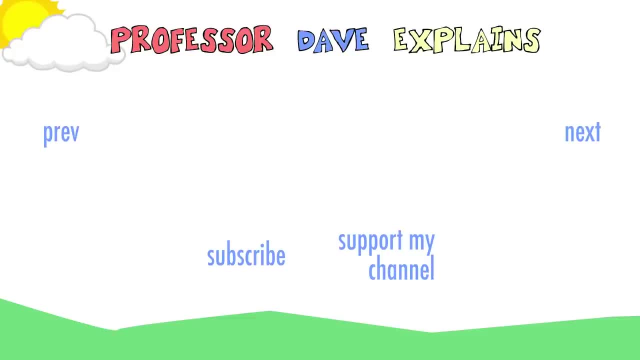 me. Thanks for watching and I'll see you in the next one. I'll see you in the next one: Peace, Peace, Peace, Peace, Peace, Peace Peace.